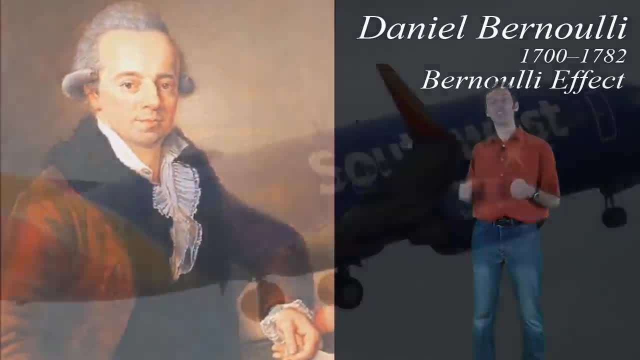 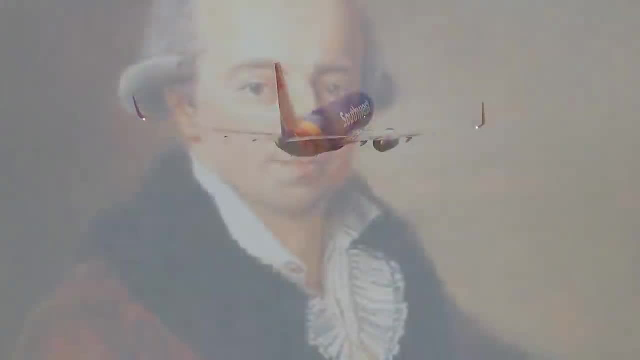 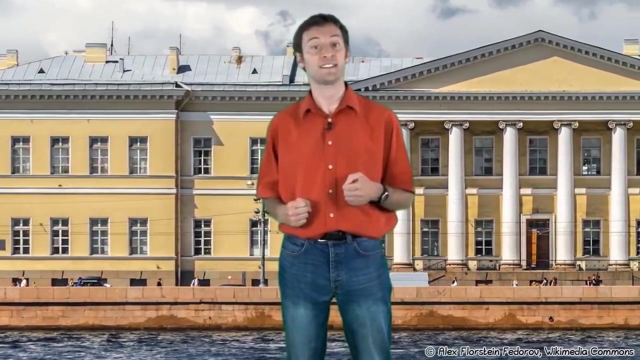 as it was one of their number, Daniel, who would go on to describe what is now known as the Bernoulli effect, the principle that enables aircraft to fly. It was Daniel Bernoulli who, in 1727, secured Euler a post at the Imperial Russian Academy of Sciences in St Petersburg. 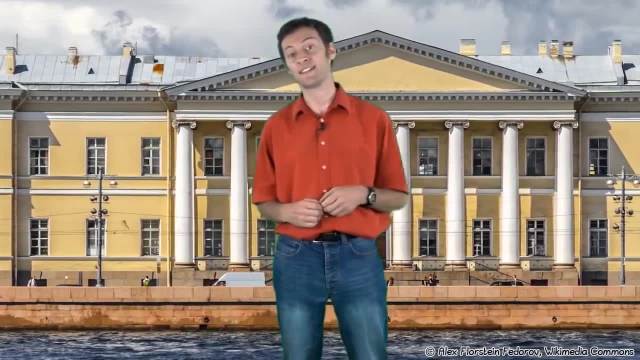 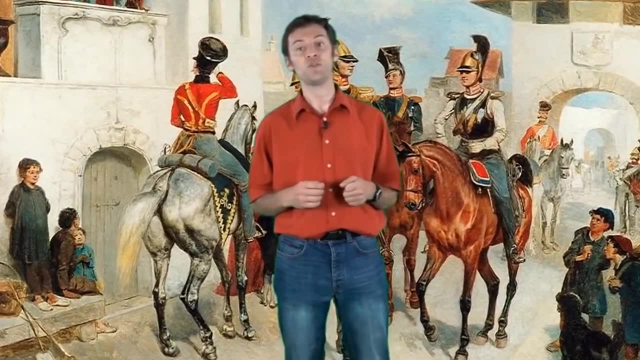 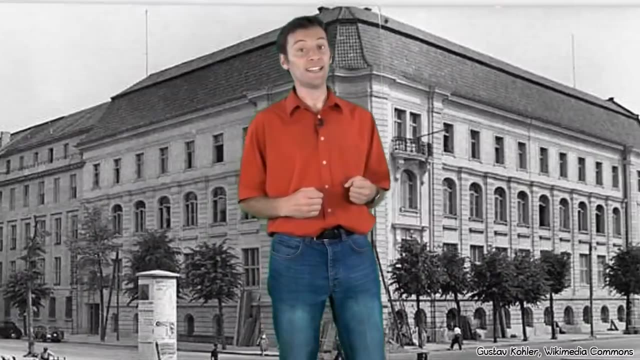 Euler would eventually replace Bernoulli as the head of the mathematics department, but, concerned about the continuing turmoil in Russia, Euler left St Petersburg in 1741 to take up a post at the Berlin Academy. It was while Euler was in Berlin that he published his Introduction to Analysis of the Infinite. 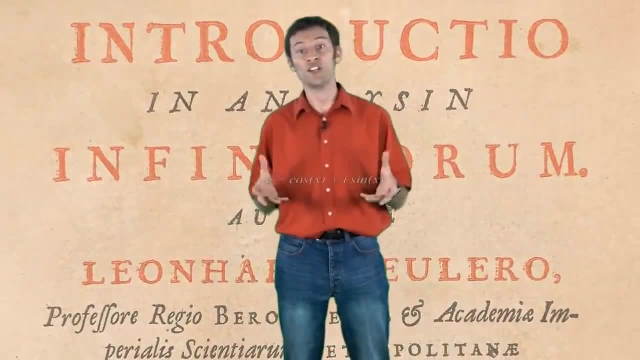 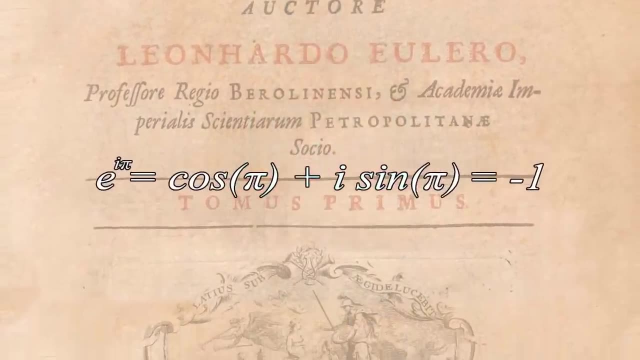 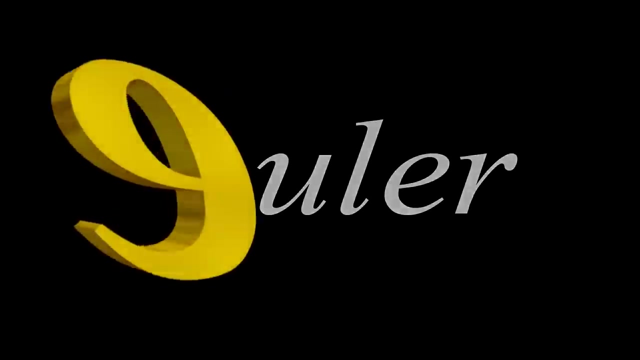 in which he expressed what is now known as Euler's formula, a special case of which led to Euler's identity. Strangely enough, the special number E, known as Euler's number and used in Euler's formula, was not actually discovered by Euler himself. 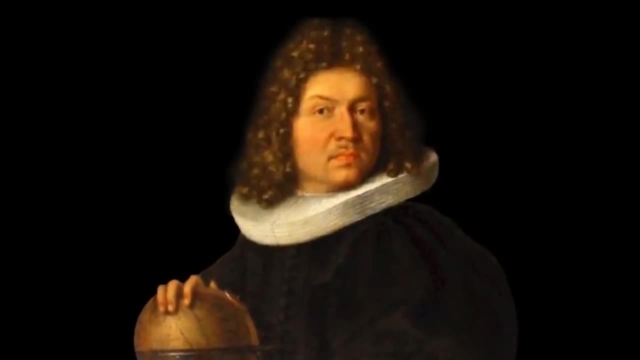 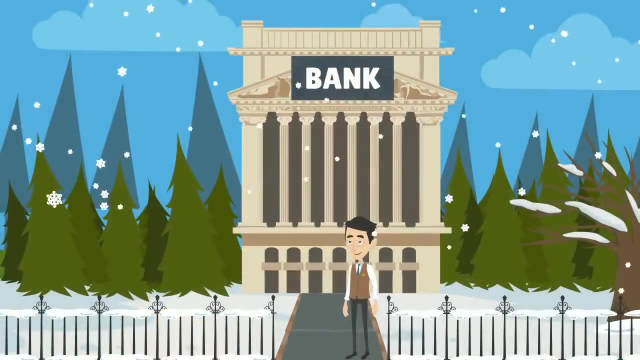 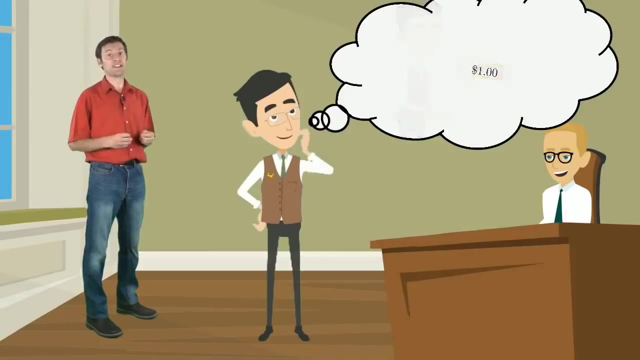 It was discovered instead by another of the Bernoulli clan, Jacob Bernoulli, who came across it whilst working on the principle of compound interest. Jacob Bernoulli found that if he deposited one dollar at the beginning of the year and awarded himself a total of 100% interest over that year, 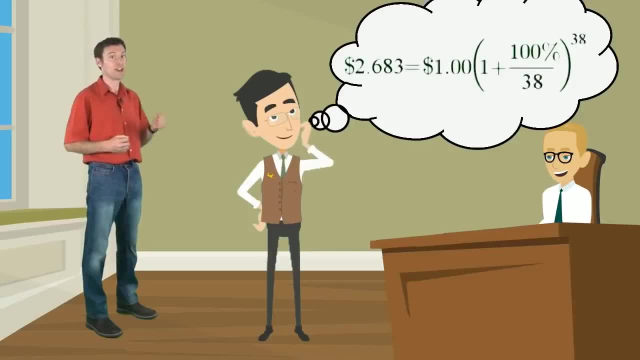 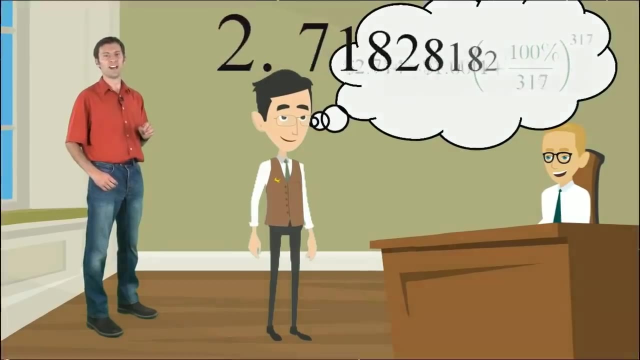 no matter how many times he divided the interest payments throughout the year, he couldn't get past a grand total of $2.72 by the end of the year. The exact number is actually 2.718281828459045235360287471. 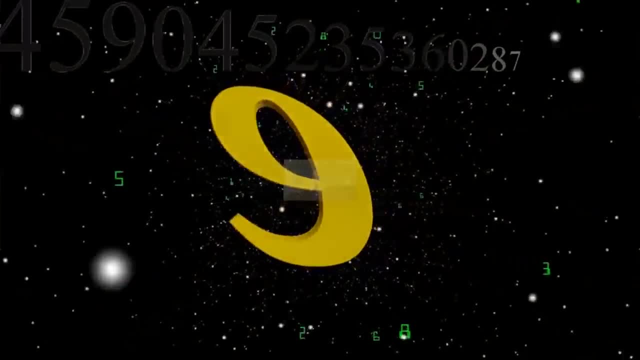 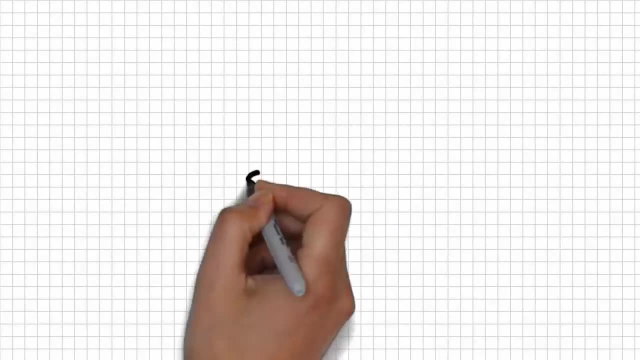 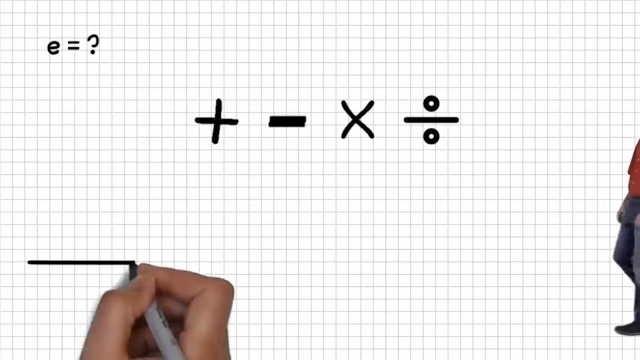 It was Euler who named this number E after his own name, and that has been the symbol that has stuck. But how is E actually calculated? The humble calculator knows only four mathematical operations: addition, subtraction, multiplication and division. The number E can actually be calculated by an infinite series. 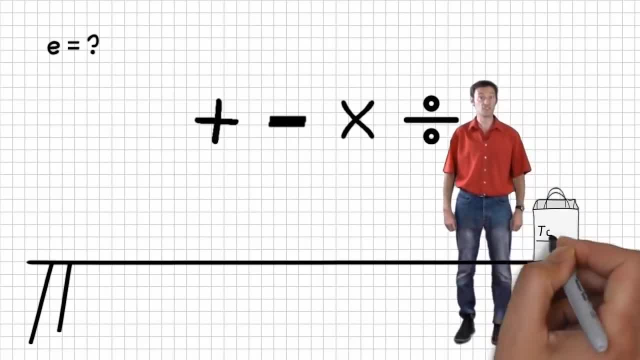 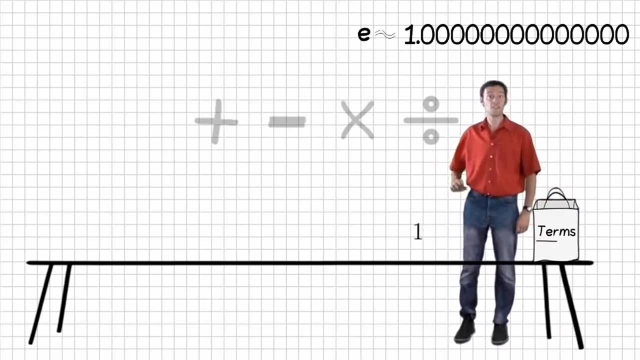 of additions, multiplications and divisions like this: We start with 1.. To this we add 1 divided by 1 factorial. This gives us 2.. We then add 1 divided by 1 times 2, otherwise known as 2 factorial. 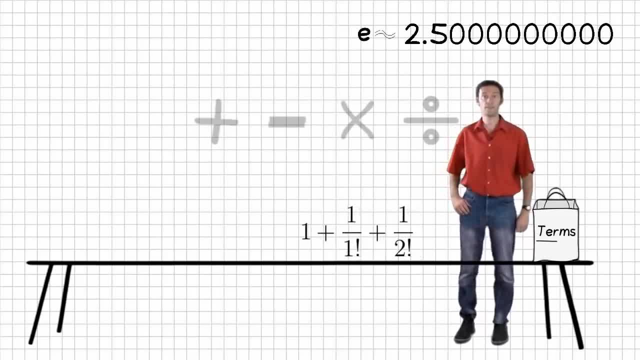 This gives us 2.5.. We then add 1 divided by 1 times 2 times 3, or 3 factorial, This gives us 2.666.. We then add 1 divided by 4 factorial, This gives us 2.708.. 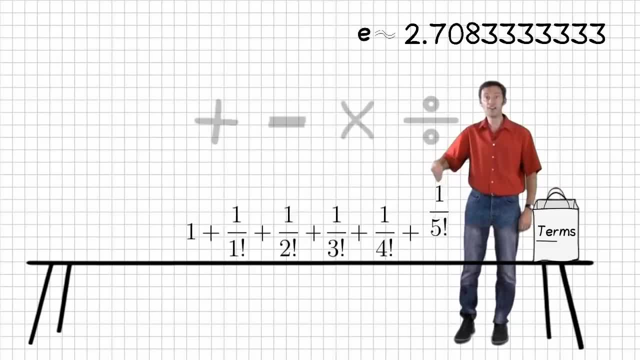 We then add 1 divided by 5 factorial, This gives us 2.716.. As we add more and more terms into the equation, we get closer to the precise value of Euler's number. The beautiful thing about this equation is that it is very easy. 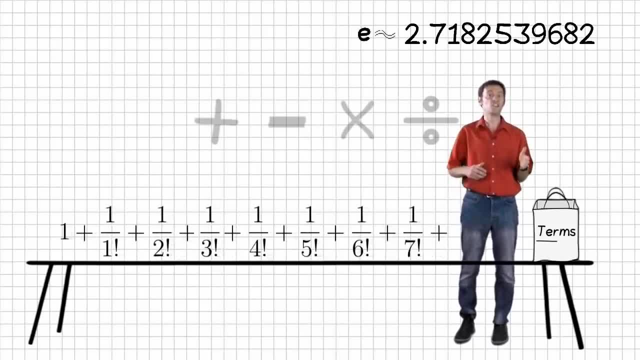 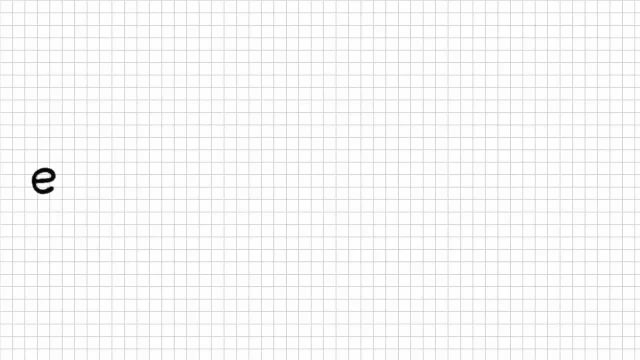 to predict what the next term will be, as each time the denominator factorial is increasing by 1.. Now E, as we have written it here, is like writing E to the power of 1. If we wanted to make this more general and raise E to the power of x, 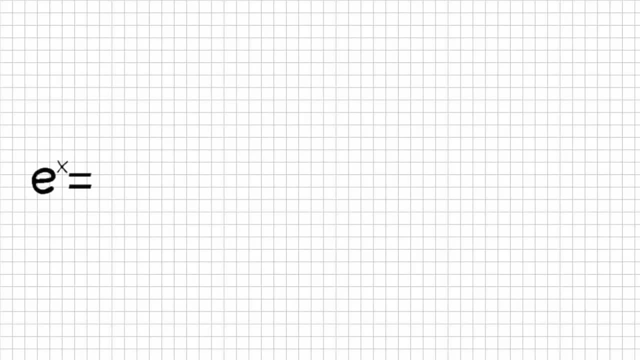 then the infinite series changes to 1 plus x over 1 factorial plus x squared over 2 factorial plus x, cubed over 3 factorial, plus x to the 4 over 4 factorial, and so on. Now it just so happens that E to the x is not the only thing. 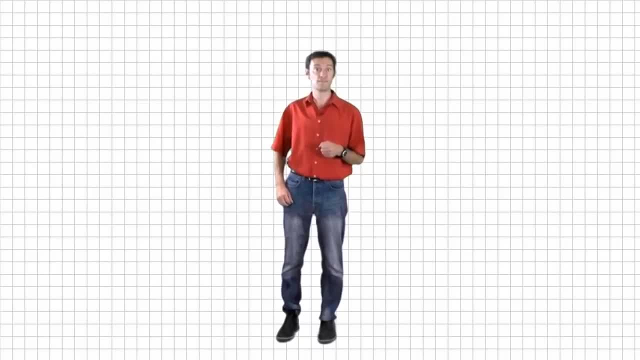 that can be calculated by such an infinite series. The trigonometric functions sine and cosine can also be calculated by infinite series. Sine of x is equal to x divided by 1 factorial minus x. cubed over 3 factorial plus x to the 5 over 5 factorial. 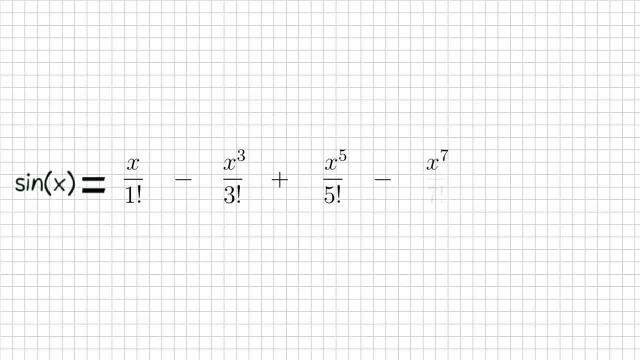 minus x, to the 7 over 7, factorial, and so on. Again, it's easy to predict the continuation of this series, as each time the denominator is increasing by 2, as is the power to which we are raising x, The sine of each term keeps alternating between a plus and a minus. 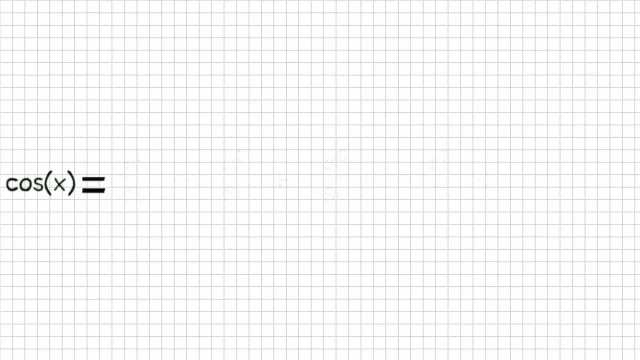 Something similar happens with the cosine of x too: 1 minus x squared over 2 factorial plus x to the 4 over 4 factorial. minus x to the 6 over 6 factorial plus x to the 8 over 8 factorial, and so on. 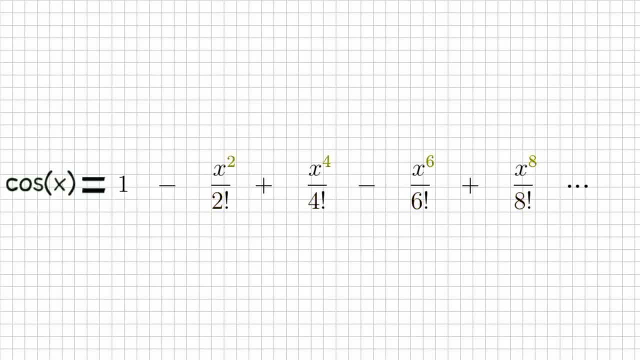 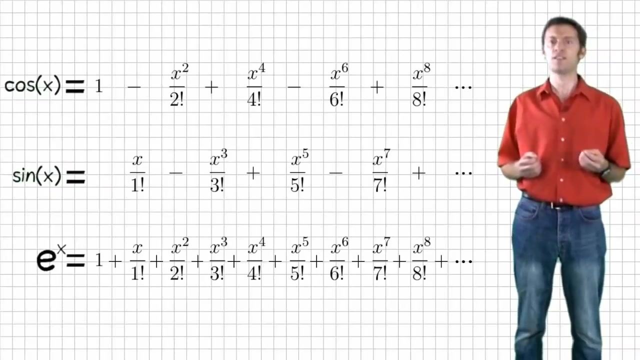 Again, like the sine series, the denominator and power terms increase by 2 each time. only this time, instead of starting from 1, they begin from 2.. The infinite series for cosine, sine and E look so similar to each other. 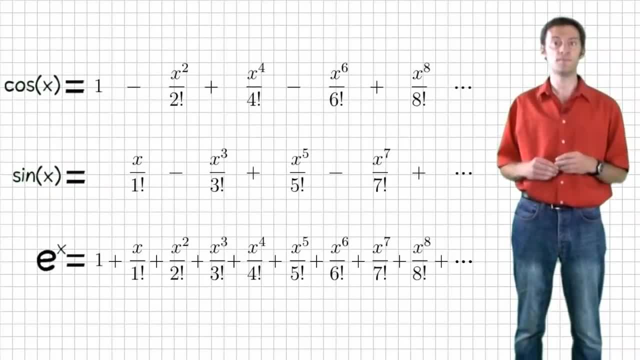 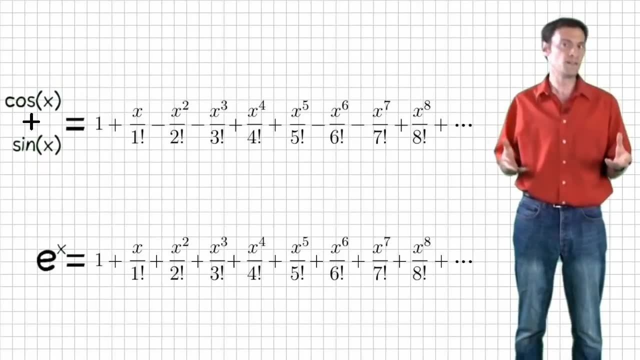 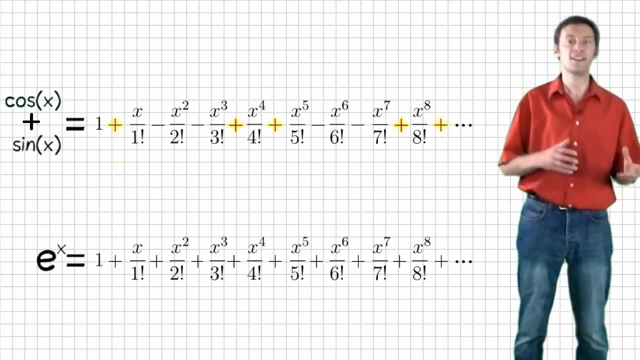 that you might be forgiven for thinking that there is a relationship between them. If we were to add the cosine and sine series together, would that give us Euler's number? Well, unfortunately not. There's a little problem. The problem is that the signs between the terms 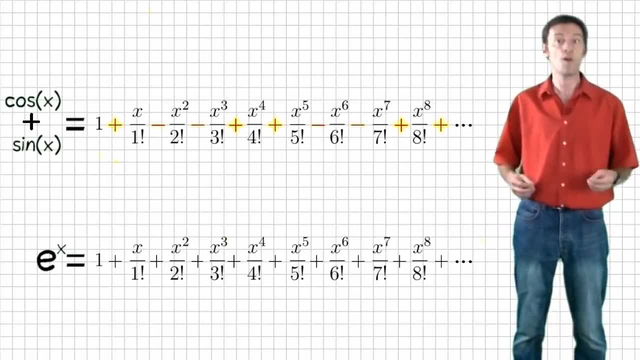 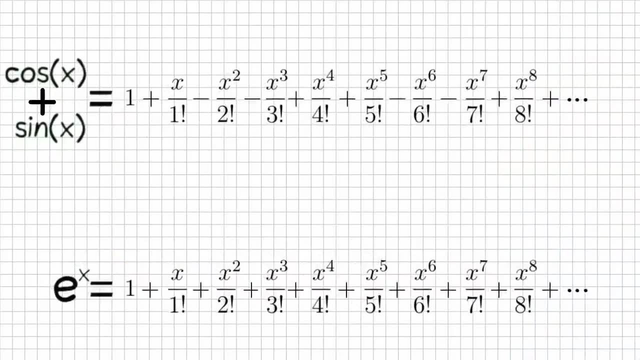 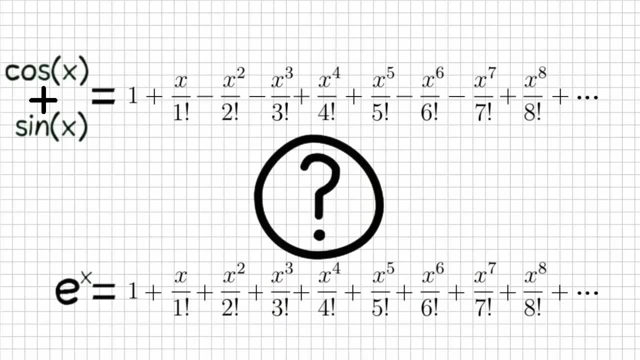 in the sine and cosine series keep changing, whereas in the series which calculates Euler's number they don't. If only there was some way we could sort out this series, some number. we could multiply the x term by to make the two equations equal each other. 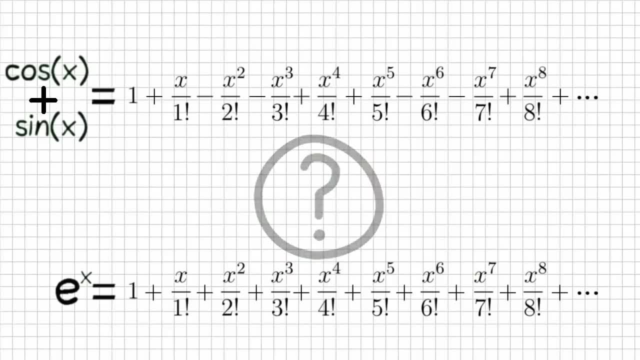 In order to make the equations equal, there's something we would need to. multiply x by when it was squared would have to equal minus 1.. The same would be true when x was cubed again, when x was raised to the power of 6 and 7, and so on. 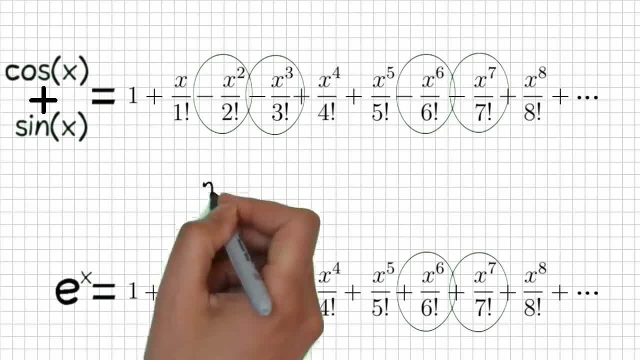 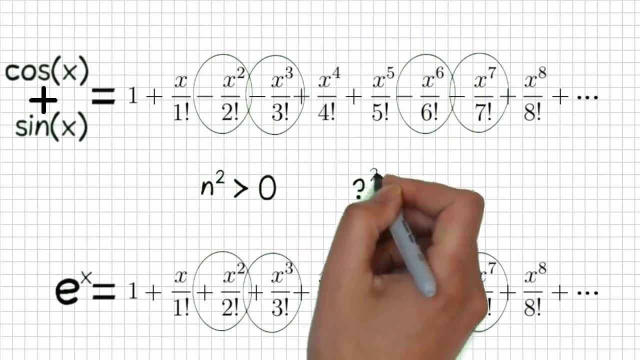 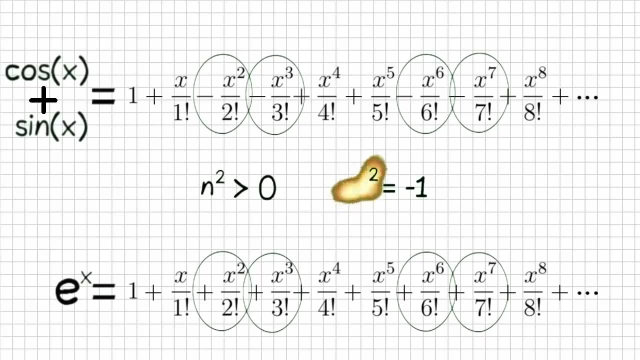 The problem is: when we square a number, the result is always positive, not negative. What we need is a number that, when squared, is equal to minus 1.. The problem is, such a number doesn't exist. The brilliant thing about mathematicians: 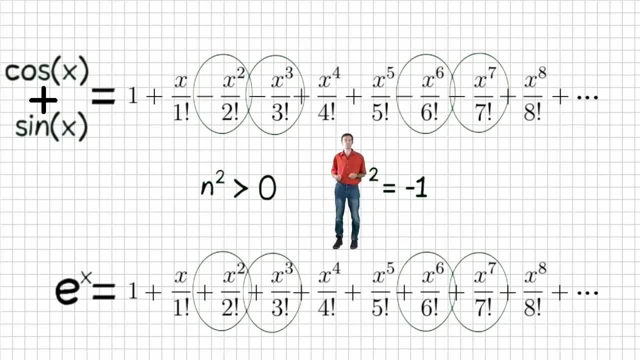 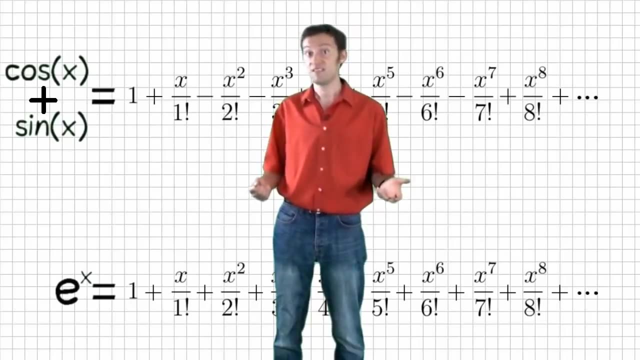 is that, when they're on their way to some wonderful mathematical discovery, they don't let a little thing like numbers not existing stop them. After all, mathematics is the science of numbers. so if a number, rather inconveniently, doesn't exist, well, they just jolly well go out and invent one. 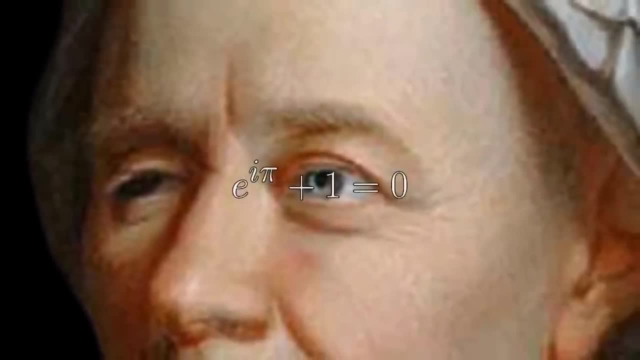 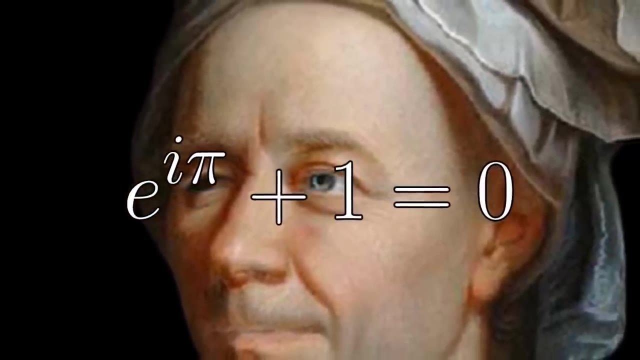 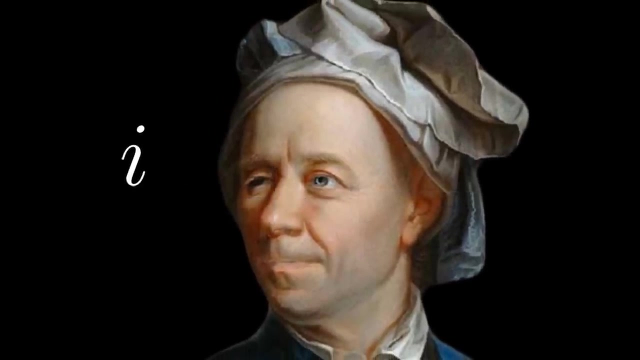 As it happens, Euler's identity wasn't the only place where it would have been useful to have a squared number equally minus 1.. The same problem was happening all over mathematics, And so was born the imaginary number i. i is the only number that, when squared, 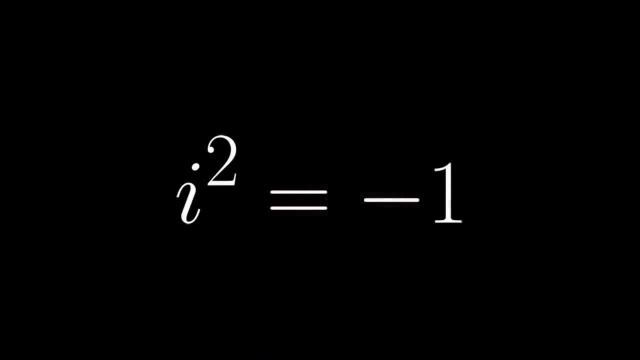 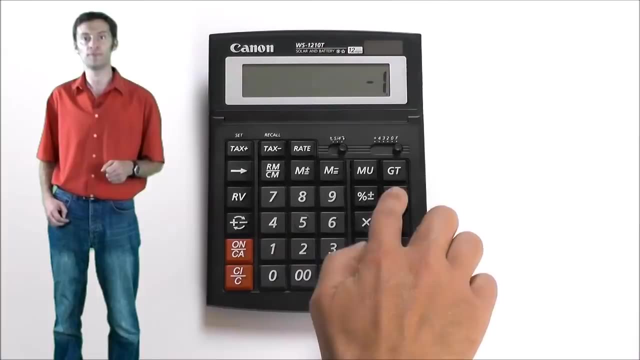 gives us a negative result, namely minus 1.. By now you might have tried plugging the number minus 1 into your calculator and hit the square root button. Your calculator, unless it's a very clever one, will have gallantly refused to give you an answer. 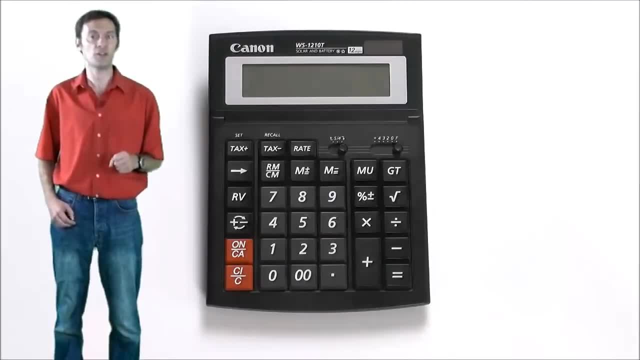 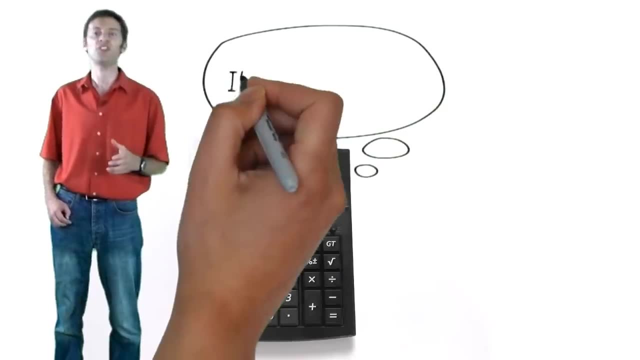 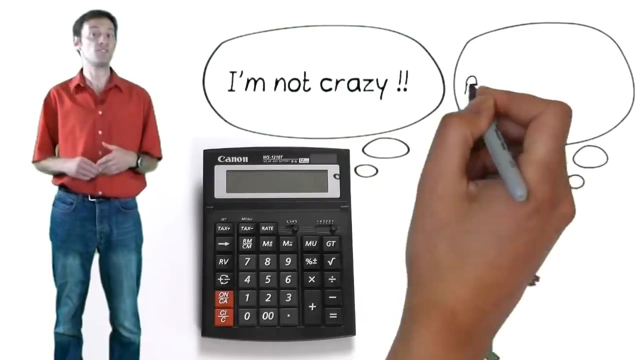 Maybe the word error is currently showing on its readout. That's because your calculator is a rational piece of electronics and cannot deal with numbers which don't exist. However, in the eyes of a mathematician, just because a number doesn't exist doesn't mean that it cannot be useful. 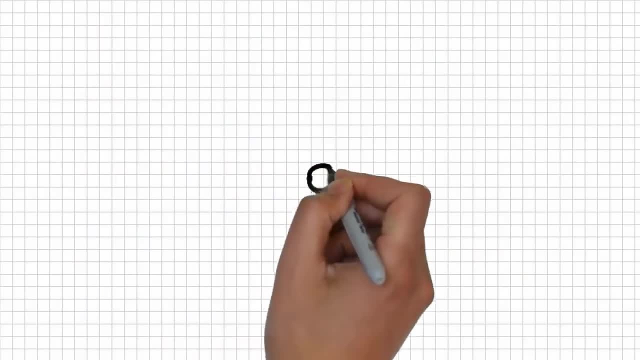 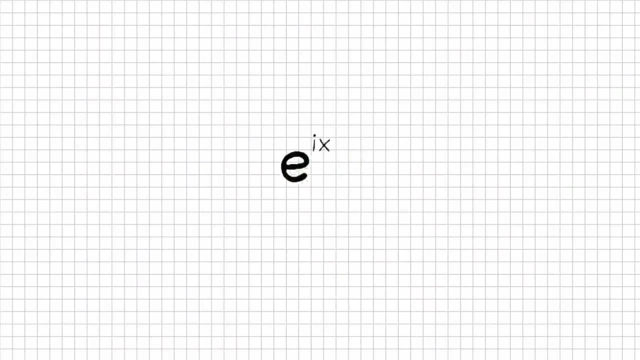 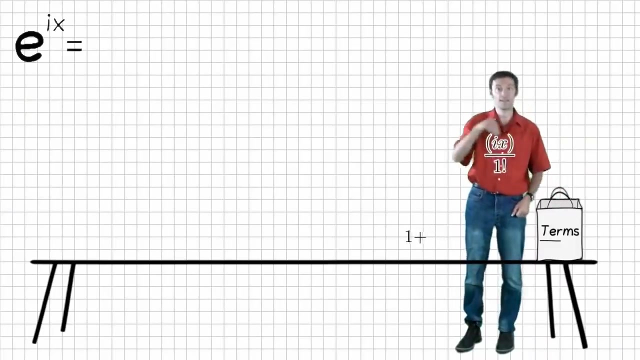 What happens if we take Euler's number and raise it not to the power of x but to the power of i, the square root of minus 1, times x. This will give us 1 plus ix plus ix squared over 2. factorial. 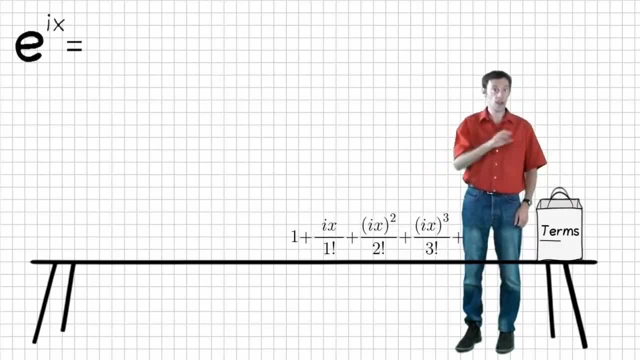 plus ix cubed over 3 factorial, plus ix to the 4 over 4 factorial, and so on. But we just said that i is the square root of minus 1, therefore if we square it, we'll just get minus 1.. 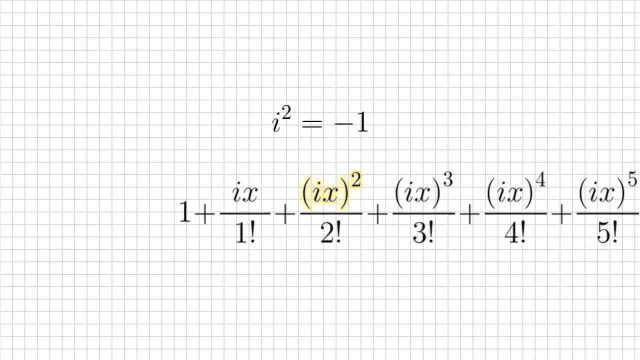 Just look at that term over there. There we have ix squared, So we could rewrite those brackets as minus x squared. Now i cubed is the same as i squared times i, so that term can be written as i squared, which is equal to minus 1,. 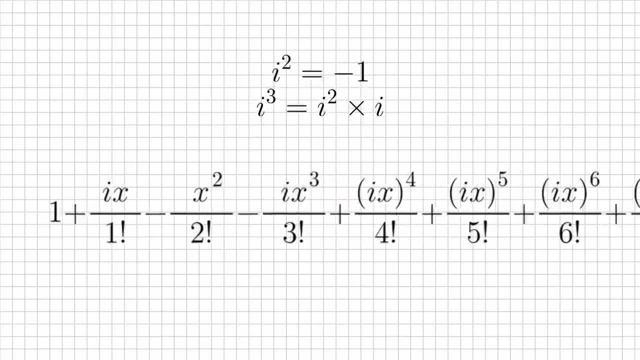 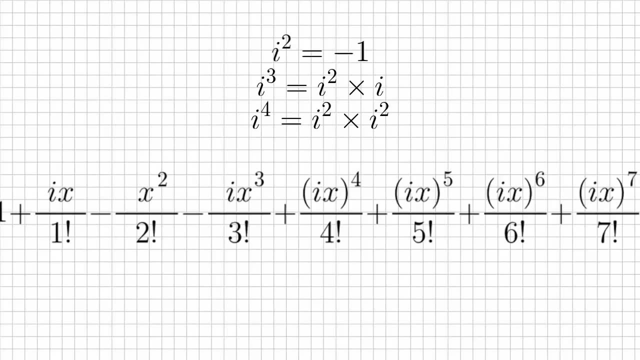 times i times x cubed. i to the power of x, i to the power of 4, is the same as writing: i squared times i squared. so minus 1 times minus 1 equals 1.. So that term there is just x to the power of 4.. 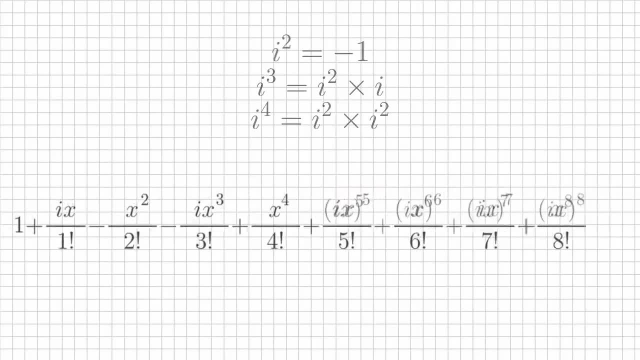 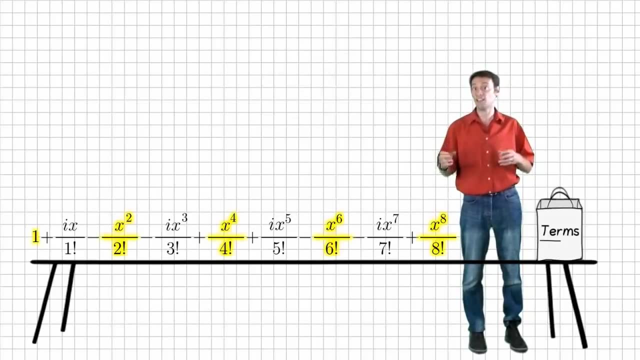 This is beginning to look like the series we worked out before for cosine of x plus sine of x. Now we have some terms that are real, ie they're not multiplied by i, and some terms that are imaginary- The terms that are multiplied by i. 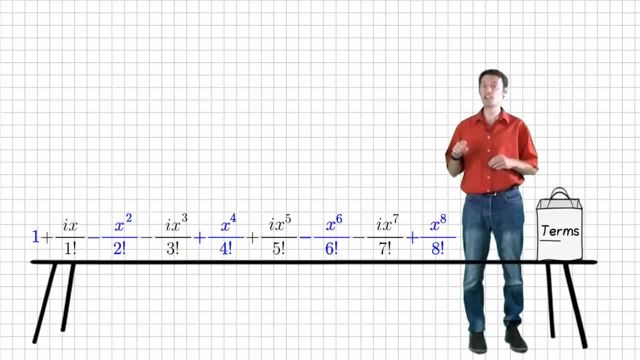 Let's highlight the real terms in blue and the imaginary terms in red. Now let's move everything around so that we group the real and imaginary terms together. All the imaginary terms are multiplied by i, so we can factor i out. Now the real terms are the terms. 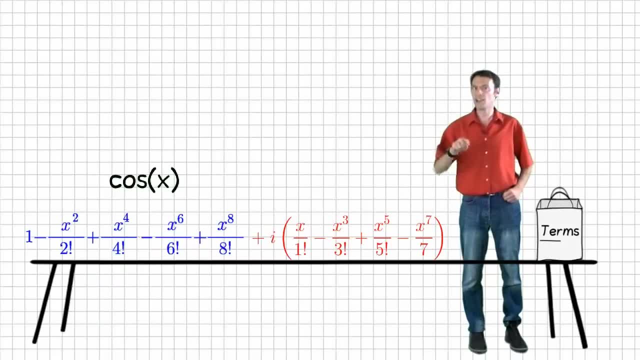 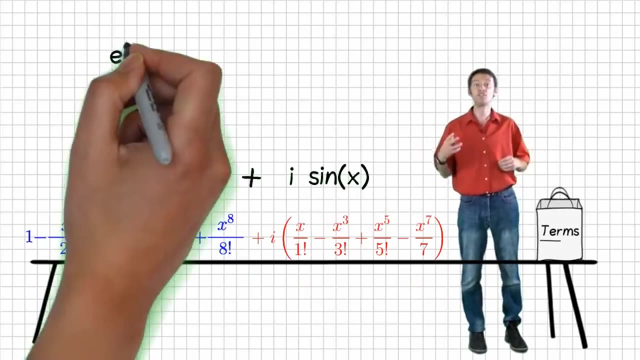 we use to calculate cosine of x and the imaginary terms are the terms we use to calculate sine of x. It's just we've multiplied them all by i, So there is a relationship between Euler's number and cosine and sine. It's just that we have to raise e to the power of ix. 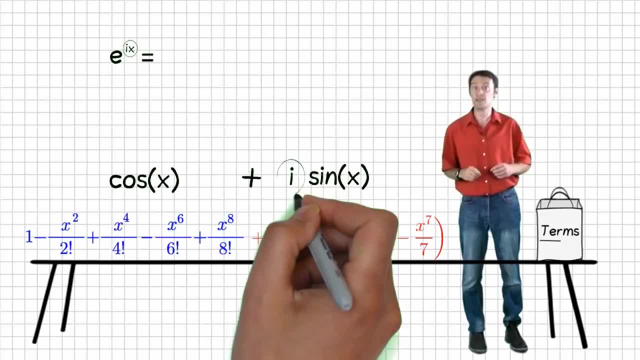 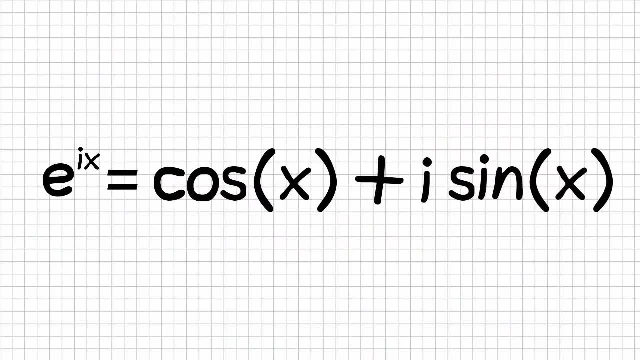 and multiply the sine term by i in order to make the maths work. This is Euler's formula, which we mentioned. at the beginning of the video, I said that a special case of Euler's formula led to Euler's identity, which the physicist Richard Feynman found so beautiful. 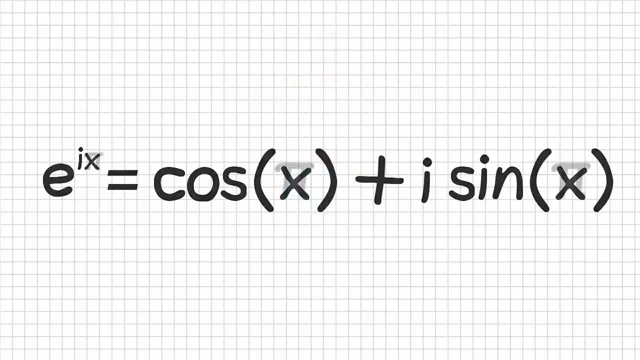 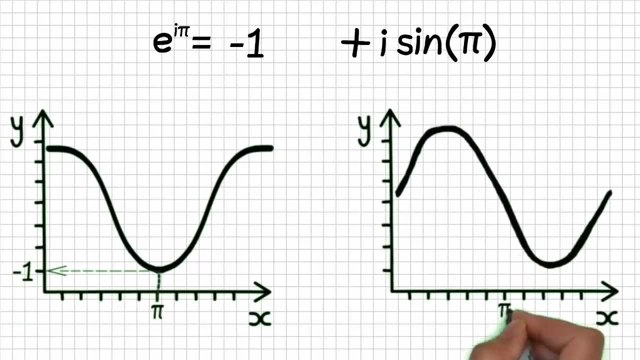 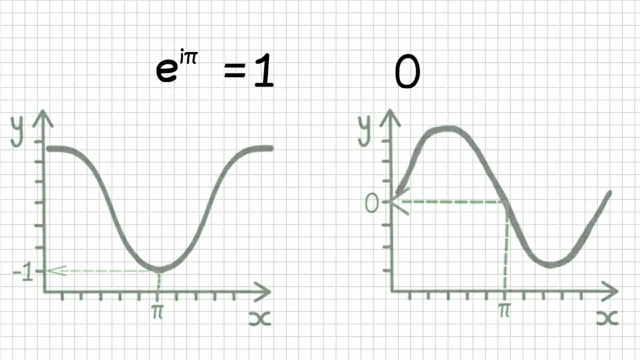 The special case occurs when x is equal to pi, Cosine of pi is equal to minus one and sine of pi is equal to zero. so e to the i, pi is equal to minus one. Rearranging this slightly gives us Euler's identity. 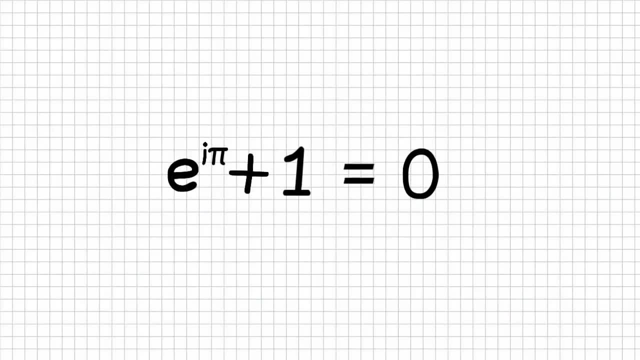 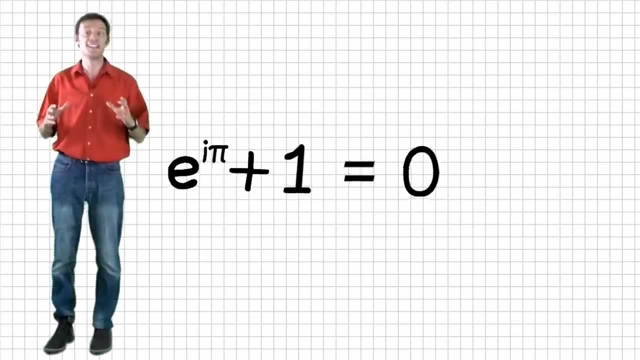 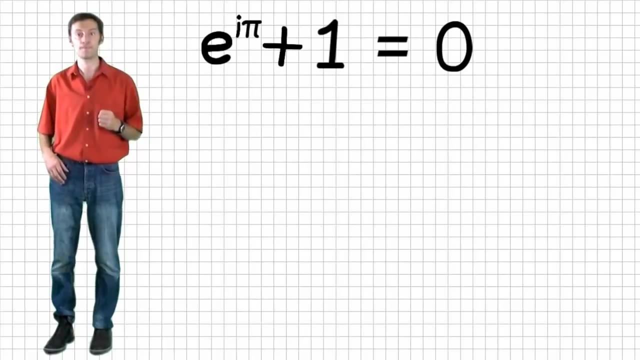 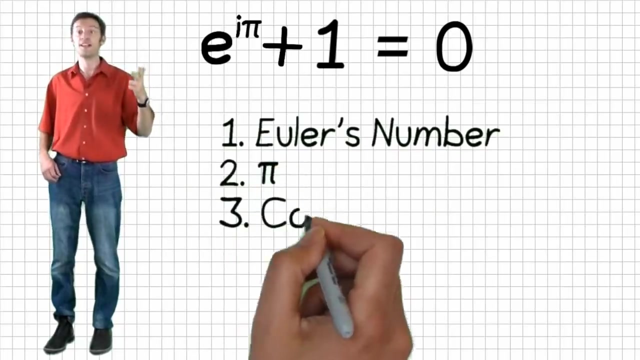 e to the. i pi plus one equals zero. What is so amazing about this little identity is that it links together in one simple relationship four completely different concepts in mathematics: Euler's number pi, the cosine and sine functions and the imaginary number i. 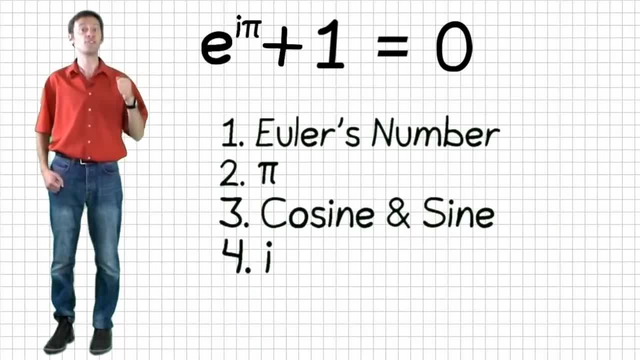 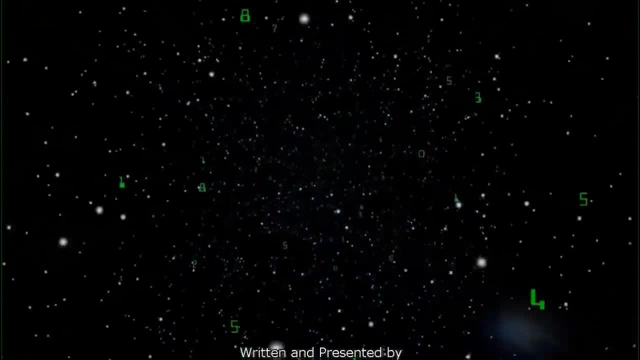 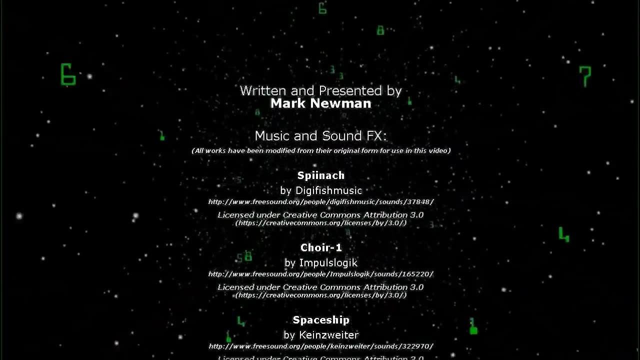 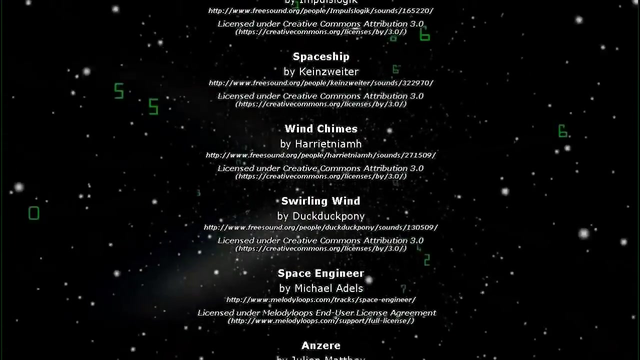 And that, in mathematical terms, is beautiful. Filming is currently underway on a special online video course which explores the Fourier transform and how it works. This video forms part of the module on: